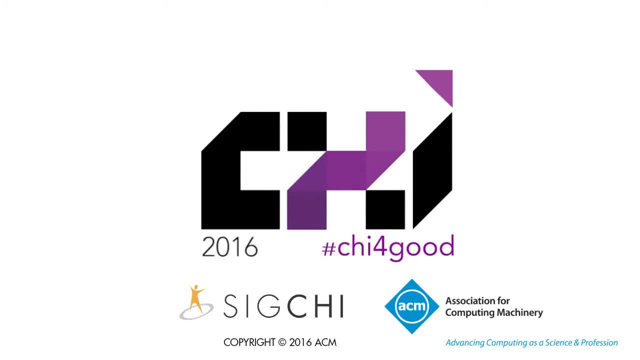 With a small exercise, I'm going to show you some claims about our field, and you have to raise your hand if you think they are true, at least partially. So please raise your hand. if you think they're true, So our field should be more scientific, Please raise your hand. 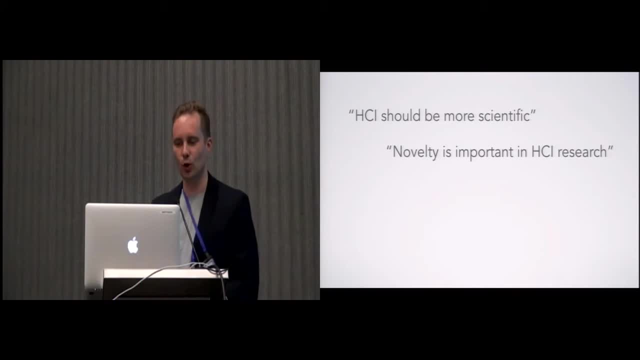 And keep your hand up. okay, So let's go to the next claim. Novelty is important in our work. Great good, A good paper reports implications to practitioners And, finally, cognitive modeling is passé. Great thanks, Kasper. what are you doing here? This talk is about belief. 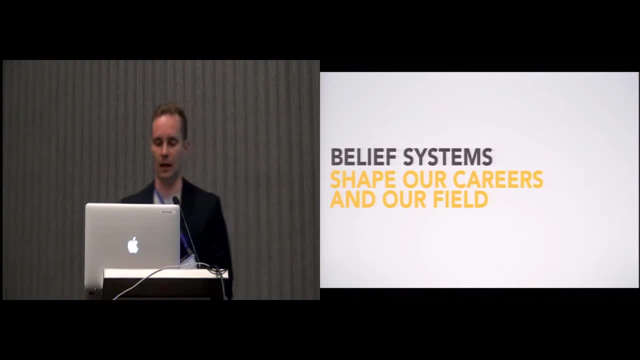 systems. So these are beliefs like the ones that you just saw, And these kind of belief systems are not like meta-theoretical claims about our field, but they are collections of beliefs that can be Not well articulated, They are not necessarily internally consistent And they don't need. 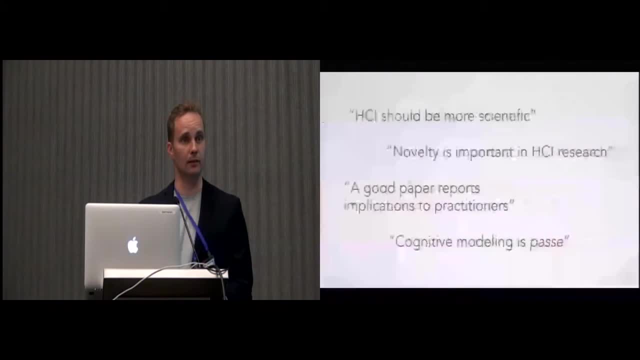 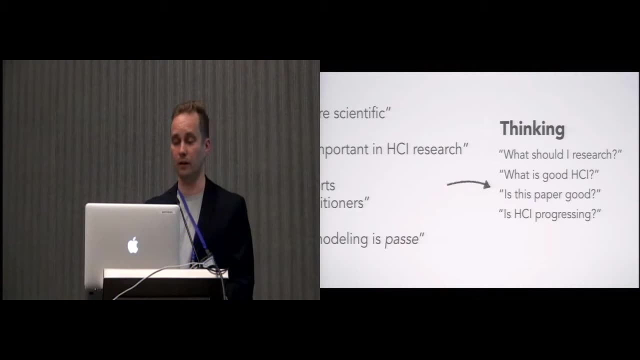 to be value-free. So beliefs like the ones that you voted for, And these are tremendously important because they guide our thinking. So, when you answer a question like what should I research? Or is this paper good, Or are we progressing on a topic? We are driven by? 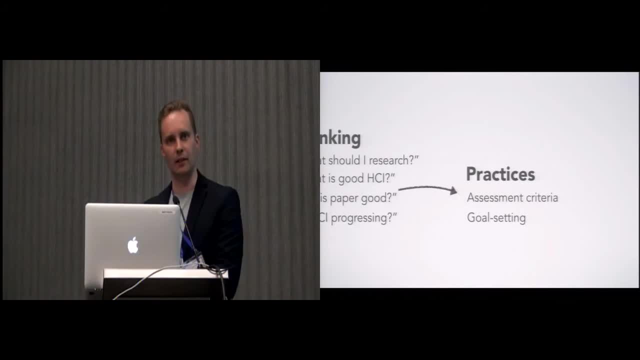 these belief systems And these belief systems, they become embodied in our practices and they become materialized. We see them in the PCM, Yes, And they are guiding our goal setting. So that's why it's really important to try to study and explicate what these belief systems are, Because if we have an ill-suited belief, 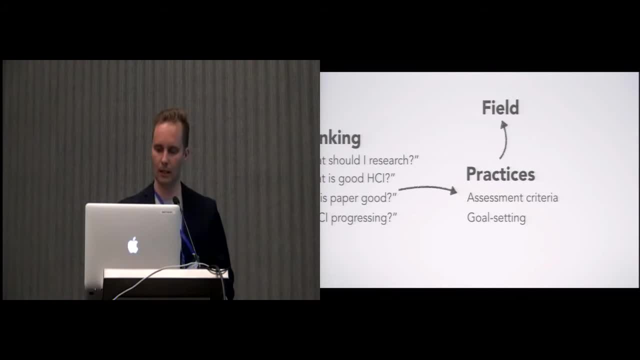 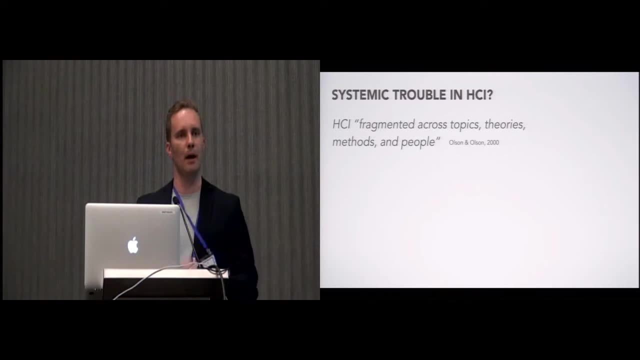 system, it can easily corrupt the whole field. Now do we have any reason to be concerned? We see really excellent work here at the conference, But if you take a step back and look at the field as a whole, here's what Olson and Olson said 16 years ago in a review paper: That 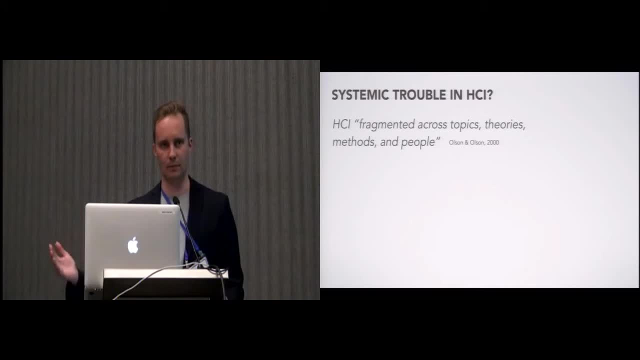 HCI is fragmented across topics and theories and methods and people. We're also noticing that there's an increasing number of disciplines contributing to our field And this means that it's harder and harder to say what is the unique role that HCI has. that doesn't 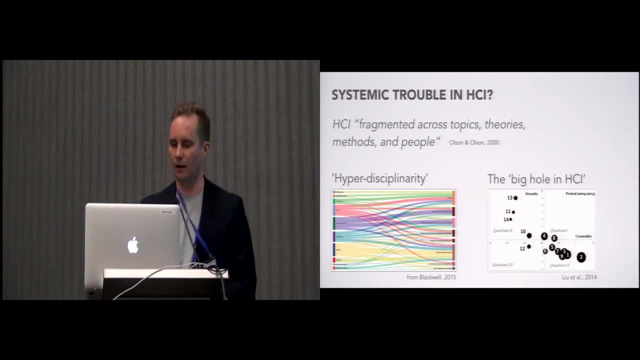 reduce back to those other disciplines. And finally, two years ago there was this argument about the big hole in HCI. In a nutshell, what it means that the results that we obtain in HCI don't drive further research in our field. So these are serious accusations. so we should be discussing what to do with these problems. 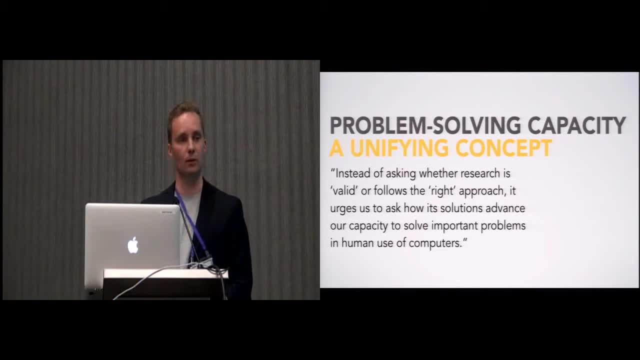 And this paper is about one such attempt, based on the problem-solving capacity, or this concept coming from Larry Lorden, And I can summarize it like this: Instead of asking whether research is valid or follows the right approach, it urges us to ask how its solutions. 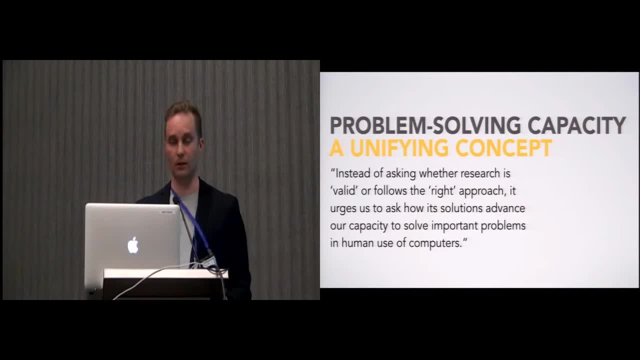 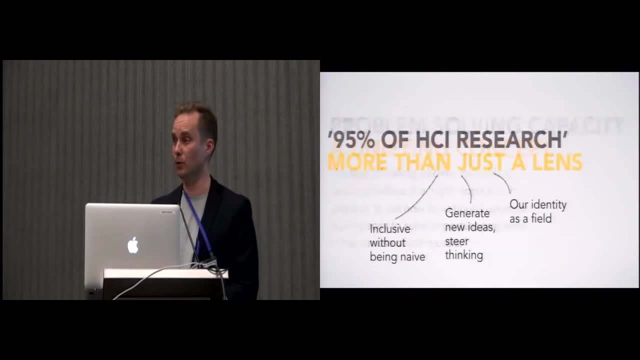 advance our capacity to solve important problems in human use of computers And we can expound this concept and use it as a lens to look at HCI. And that's what we've been doing in this paper. We try to capture the bread and butter of HCI, the kind. 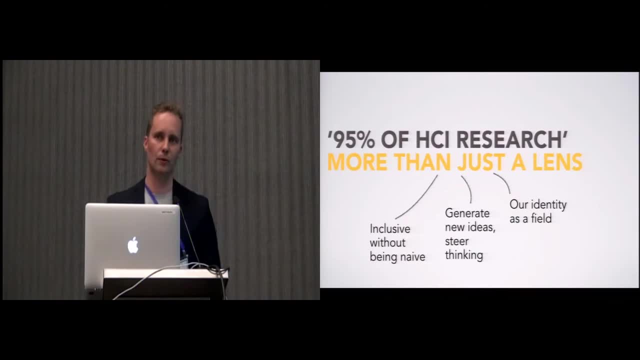 of work that you see here at the conference And to offer something more than just a lens. we're describing our identity as a field, We're offering a tool for generating and refining research ideas, And we also try to be inclusive. So try to be inclusive in the sense that we 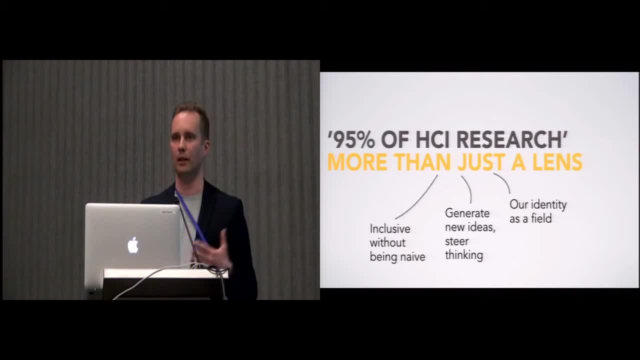 have fantastic work looking at fabrication techniques, tinkering with different kinds of engineering methods. We have fantastic works on design and we have work on looking at sub-Saharan ICT use. So how can you be inclusive and give value to that work without being naive? Naive in the sense that assuming- 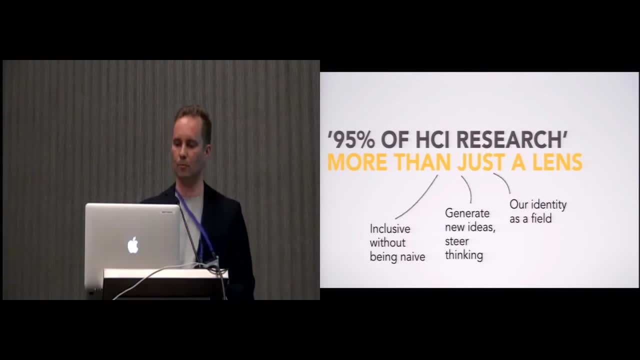 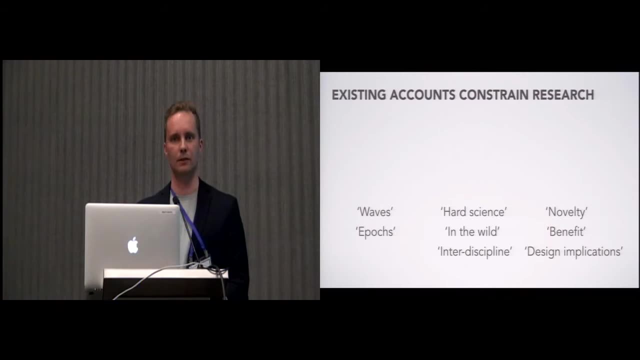 that any perspective is valuable just because it's different. Okay, A lot has been said about HCI in the past. Here's a small gallery of some of these accounts. Some of them come from real papers and some of them are in the PCS, in the review forms, And from the problem-solving perspective, they are basically filters. 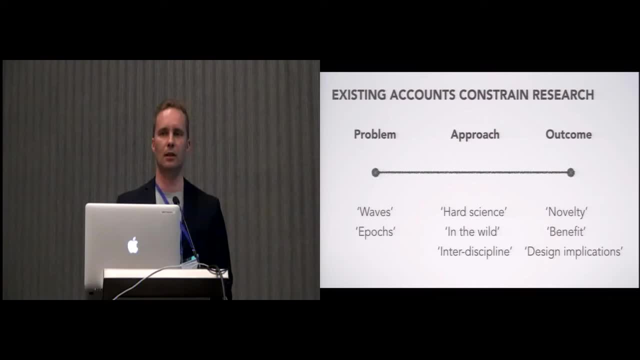 They are scoping our work. They are saying that you should not study this kind of problem or you should not use this kind of approach, or you should be pursuing this and this kind of outcome, And it's easy to come up with pretty powerful counter-examples to all of. 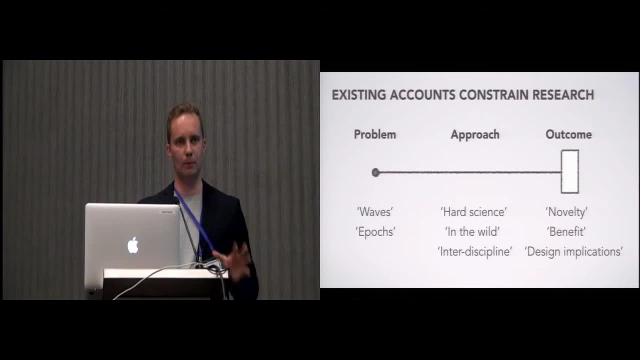 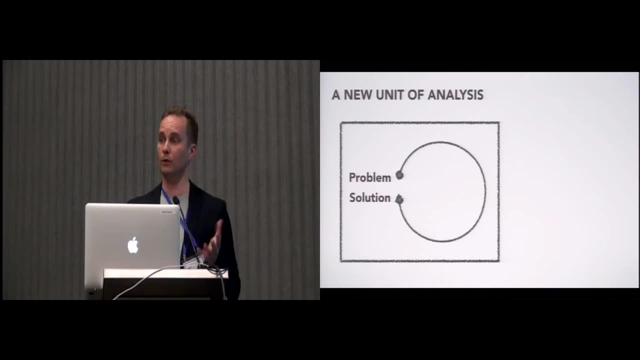 these claims And what happens with the problem-solving capacity? Here's the key idea: Instead of, we take the problem and the solution and we form a new unit of analysis called problem-solving capacity. So we ignore the approach entirely and just look at the problem and the solution. 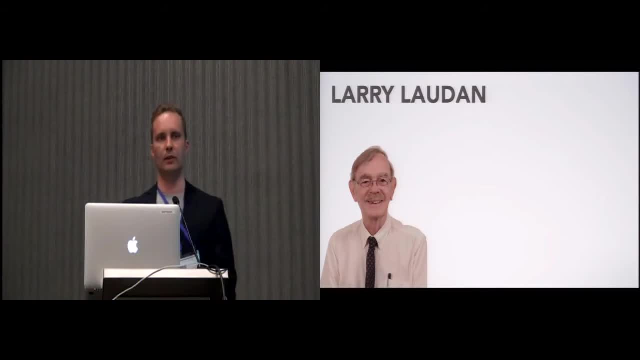 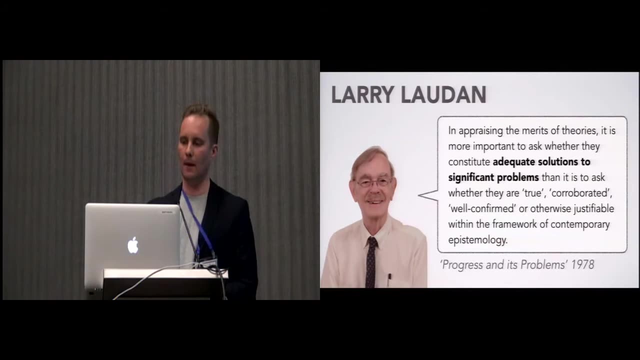 together. Now, we didn't invent this concept. It comes from Larry Laudan. He's a philosopher of science And he was debating with, for example, Kuhn, And he made this following point: In appraising the merits of theories, it is more important to ask whether they constitute. 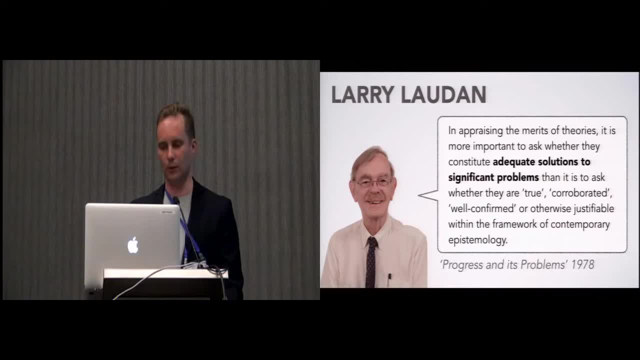 adequate solutions to significant problems than it is to ask whether they are true or otherwise justifiable within the framework of contemporary epistemology. Now we've been applying this and extending this for HCI, And the rest of the talk is about: well, what? 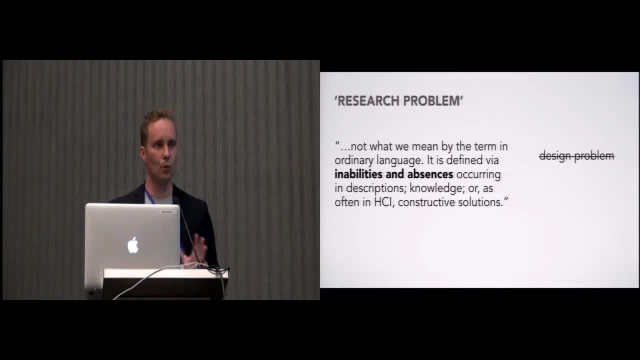 did we learn First one important point. So what Larry Laudan means by research problem is not the familiar problem as we use in colloquial language. Rather, it's defined by inabilities and absences occurring in our descriptions And knowledge And in our constructive solutions. as a field, It's not the same as a design. 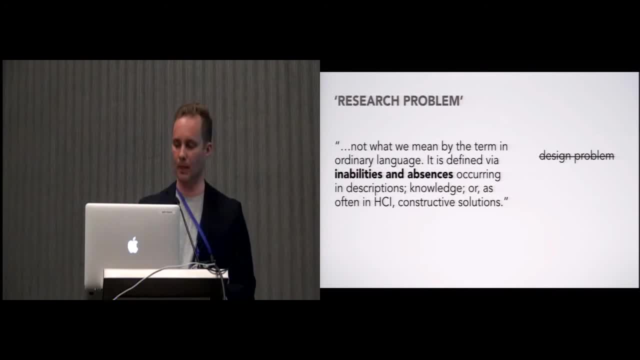 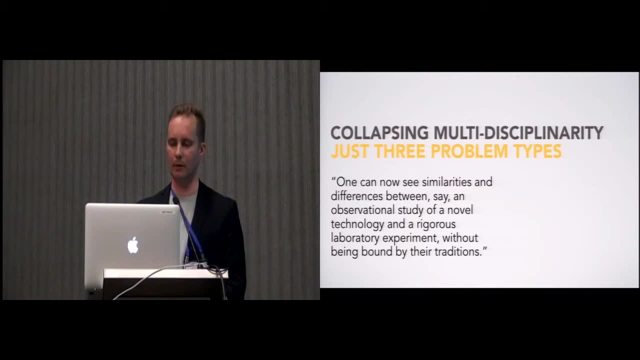 problem or a problem that a user might occur, And the first observation we did with Casper is that you can collapse this crazy hyperdisciplinary field into just three problem types And it's really valuable because you can start comparing the contributions of work coming from very 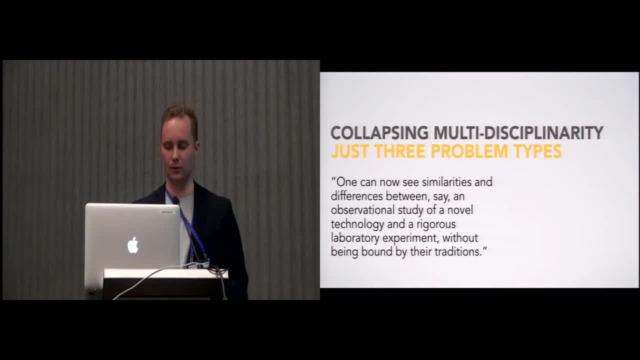 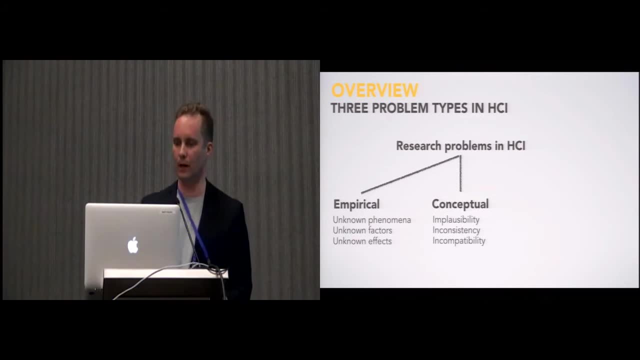 different traditions and not being bound by these traditions. So What are these three problem types? Larry Lorden introduced two of them: empirical problem type and conceptual problem type. Empirical problem type: we all know Conceptual problem type is about interrelationships between concepts. 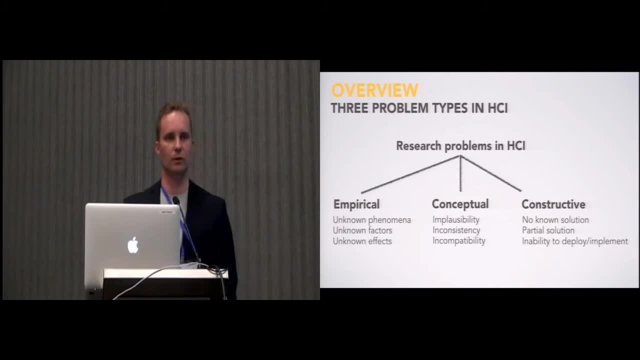 and just sort of second order problem- type And constructive problems- is something that we added with Casper, And it is basically about the construction of artifacts using, for example, means from design and engineering. What Larry Lorden also offers us is a typology. 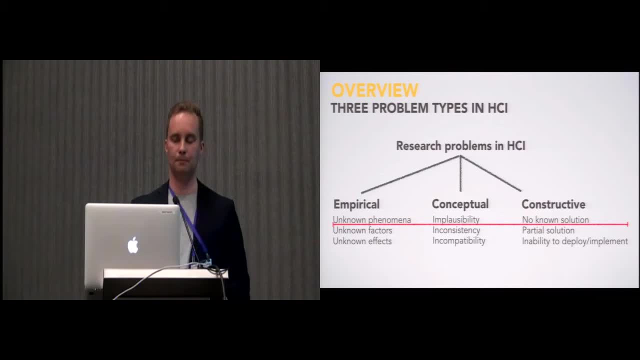 of types, of subtypes of problems, going from an increasing level of fidelity, from complete absence of description to refining and retuning these descriptions. Now we can finally try to define what problem solving capacity is, Try to show that it's something more. 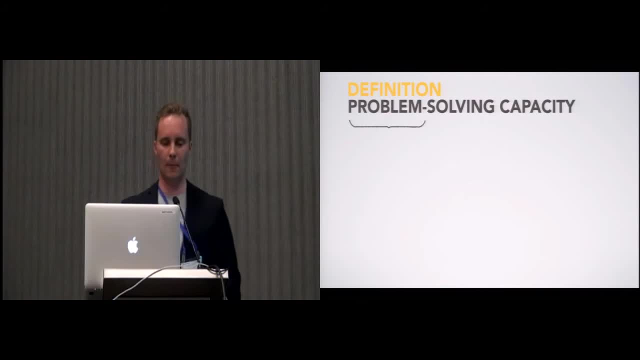 than what you typically mean by problem solving. There are five elements to this. First of all, it's about significance that we're solving significant problems related to human use of computers. This significance aspect, by the way, is often grounded to outside of our field. 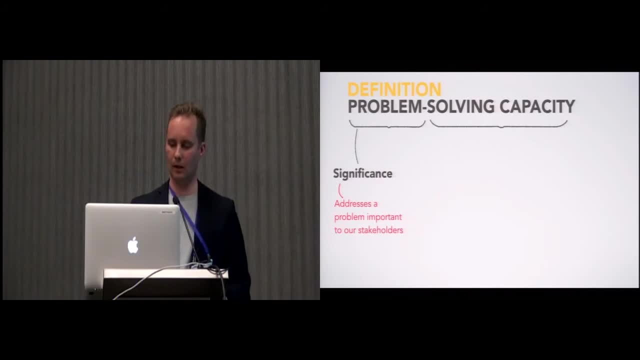 to industry and society and not necessarily to the field. It's defined by things like how many people do we address in our work or how important matters in those people's lives we address. Then there's the solution capacity aspect. that is defined in terms of three criteria. 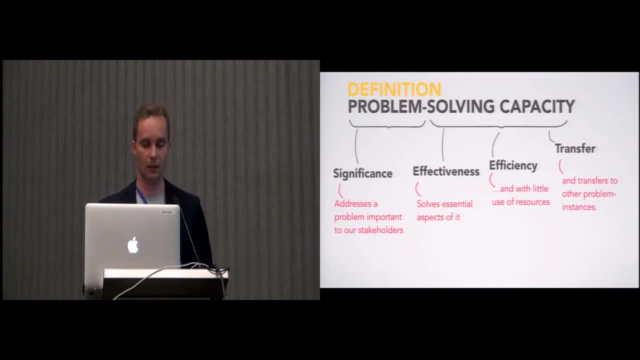 Effectiveness, efficiency and efficiency. Effectiveness, efficiency and transfer. That means that the solutions that we acquire, basically the outcomes of our work, are evaluated in terms of whether they're solving essential aspects of these problems and whether they're solved efficiently. 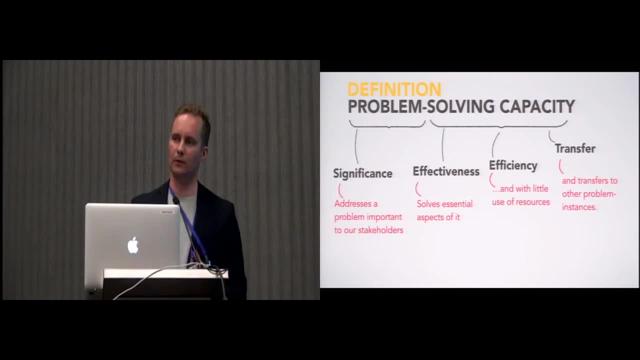 meaning with as little resource use as possible, and whether these solutions transfer from instances to another one. With Casper, we added a fifth criterion called confidence, which refers to these traditional concerns that we have about the logic of argumentation, or validity, reliability and so on. 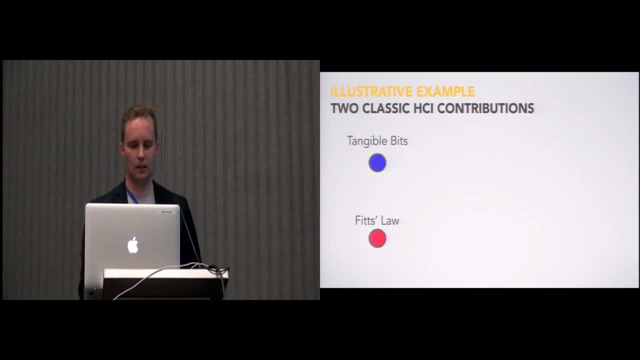 Now, this is the definition of problem-solving capacity. Now, what you can do is you can analyze your work, you can analyze whole topics in HCI, and that's what we do in the paper. And just to give you an illustration of how this works, 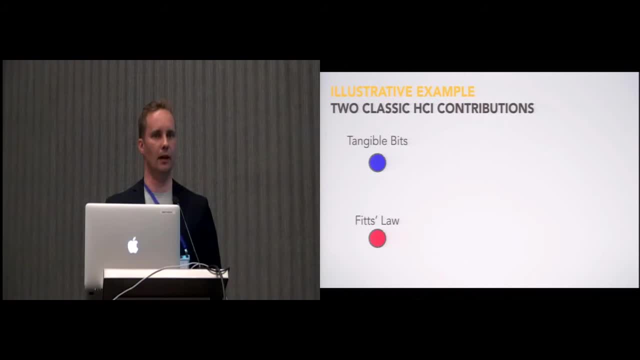 and what the benefit would be. I took two classic HCI contributions: tangible bits and Fitts' law. Normally you wouldn't even consider comparing them because they're so different. The other one is constructive, problem-type, and the other one is conceptual. 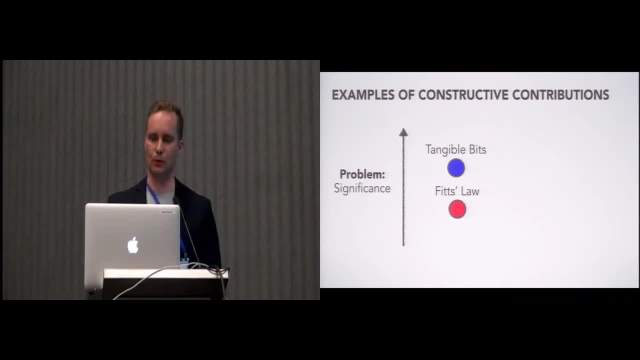 Now what do we learn if we compare that with the problem-solving capacity perspective? First of all, we should look at the significance of the problems that they're addressing And their tangible bits is better because if it would work, it would revolutionize. 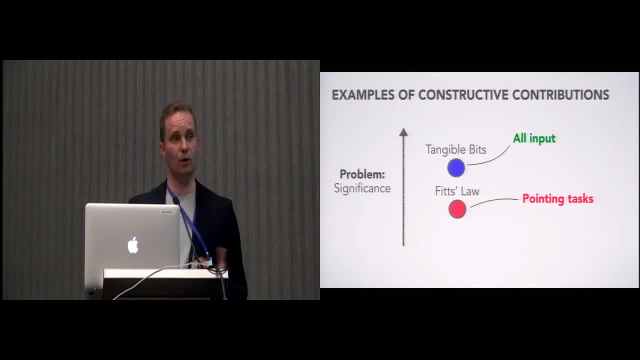 basically all of input with a computer. Fitts' law. although it's also important, it's constrained to pointing tasks. Then we also have to consider the four other criteria that are relating to the solution capacity And for the illustrative purposes. 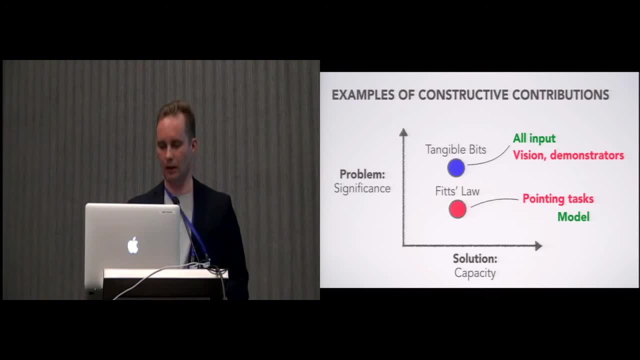 I collapsed them into just one dimension here, And how it looks like there is that this Fitts' law is stronger in that respect because it has more efficiency, effectiveness and transfer. It offers a model with which you can actually work and solve problems. 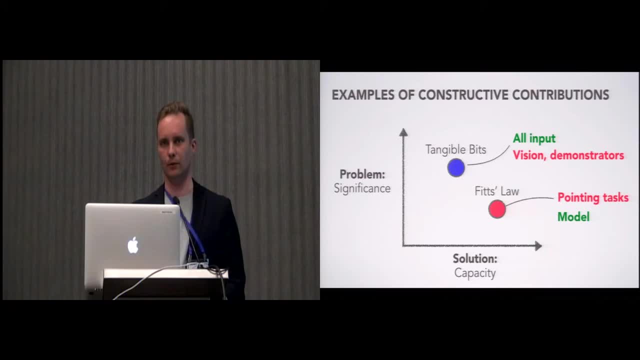 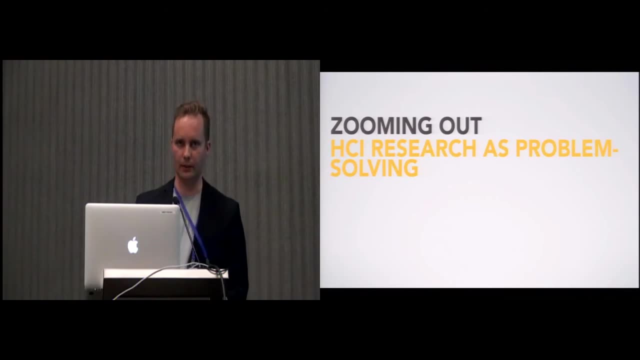 Whereas tangible bits has a vision and a set of demonstrators that are harder to then apply to different problems. Okay, so this was just an illustrative example. Now, what we wanted to learn with Casper is: what could we say about HCI as a field, as a whole? 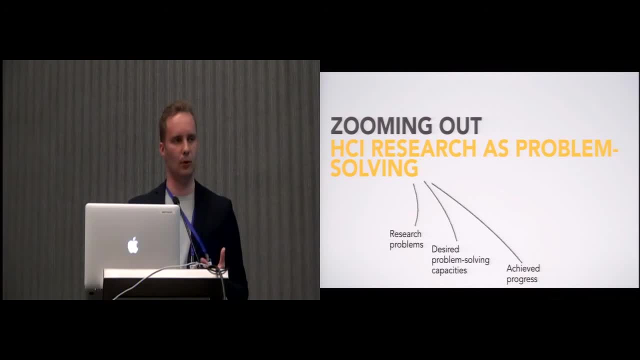 And for that end, we first had to define what it means to define a field as a problem-solving field, And it boils down to three criteria: What are the problems that we're addressing? What are the desired problem-solving capacities that we're after? 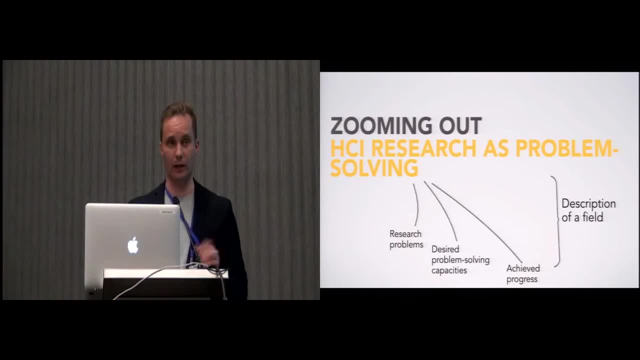 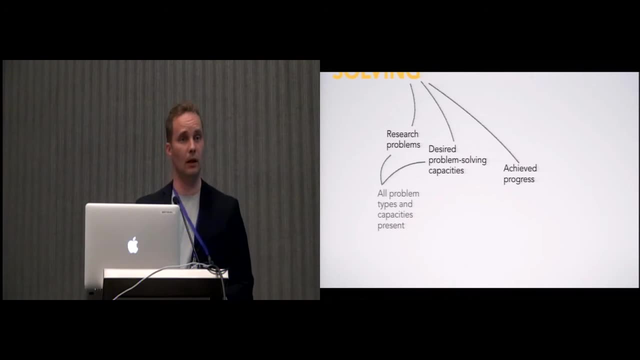 And what is the achieved progress in our work? This is a generic description of a field. Now we made some cursory first observations about HCI. First of all, that it's easy to find examples of all of these problem types and all of the capacities in HCI. 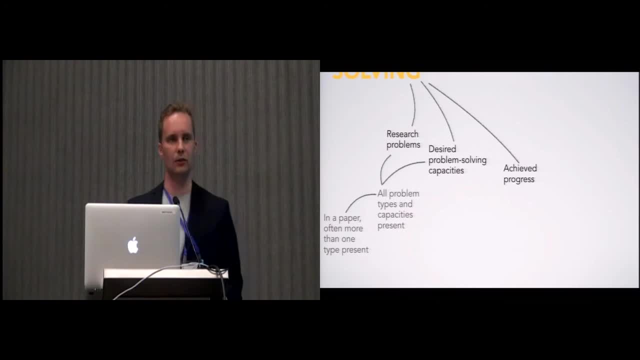 So we are really truly diverse field. In a single paper, you might easily find even two contribution or problem types, such as if you have a study and a prototype together. We seem to have high tolerance for risk, meaning that we are able to accept papers like this one. 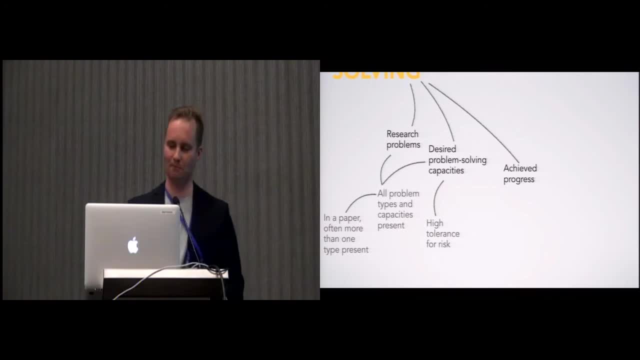 or a paper on a design, fiction or visionary paper. We also seem to ground significance not only to our own research body but to society and industry. I guess that most of you would approve with this account. And then we want to learn more and dive deeper into these papers. 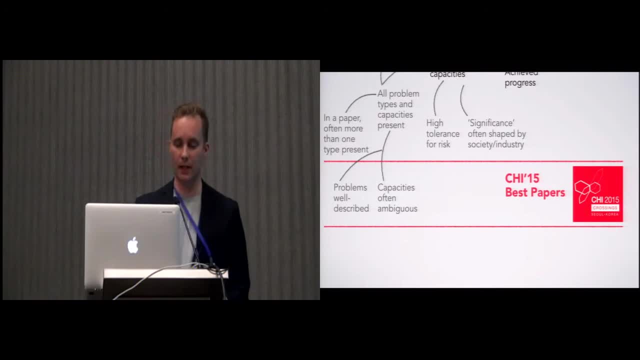 So we analyzed the best papers from last year's CHI and first made a couple of observations on how they are written, basically writing culture that we have. It seems that the problems are not the same as the problems that we have now. Okay, 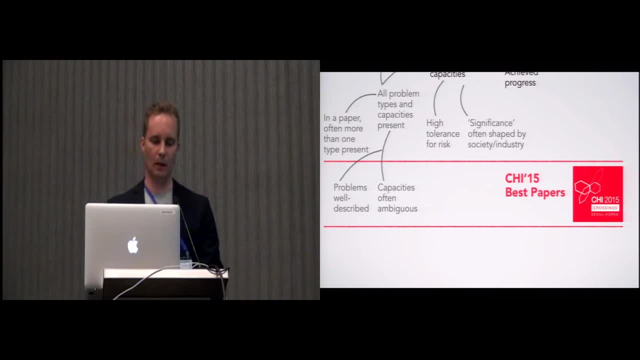 The problems per se, they are typically well-described, whereas the capacities are often ambiguously described, So we can improve in that respect. The second observation was that almost all the papers- there was only one exception- are addressing empirical and constructive problems. 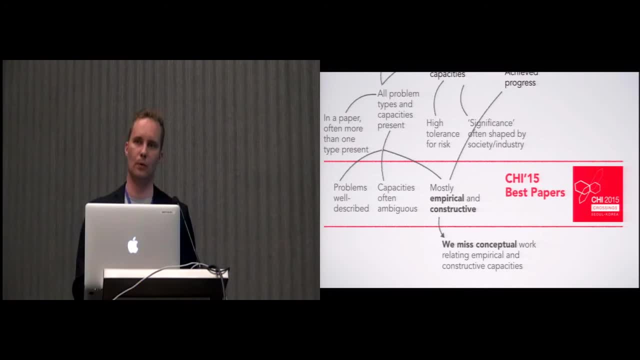 So where are all the conceptual problems? So we argue that we're missing conceptual work that is, tying together efforts in empirical domain and in the constructive domain, And this allowed us to explain why this big hole is happening. Big hole does not manifest that we are not progressing. 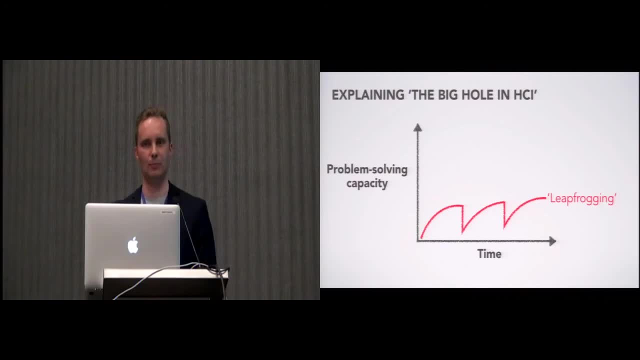 which is progressing in a particular way. that could be called leapfrogging. So whenever there's a change in technology or context, our solutions that we developed earlier don't transfer into that new setting. If we were more mature field, we would have progress like this. 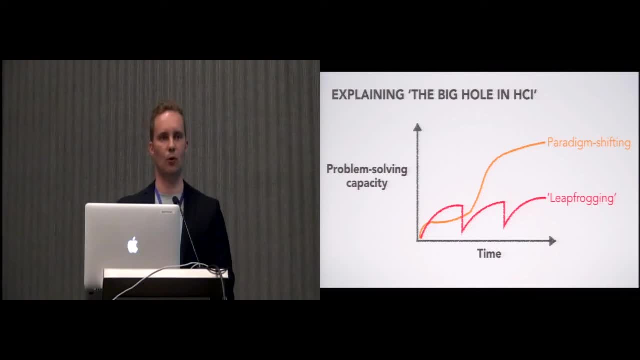 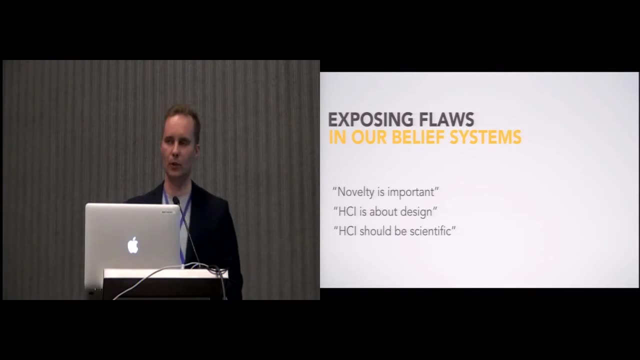 which would be initially a bit slower, but be more reliable against, or robust against, external events later on. Okay, what you can use this problem-solving view for is to expose flaws in our belief systems, to the extent that you can articulate them. 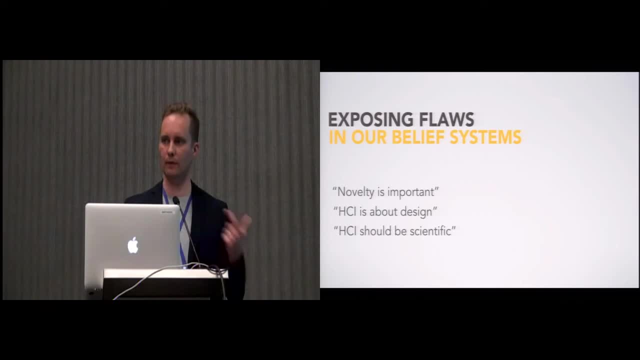 For example, the claims that we started with, And the problem-solving perspective gives you two kinds of counter-arguments to many of them: First of all, that they tend to ignore this diversity of problems and capacities we truly need in HCI, And then, secondly, many of them focus on 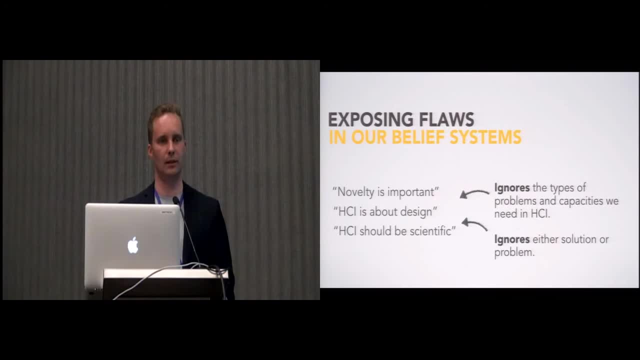 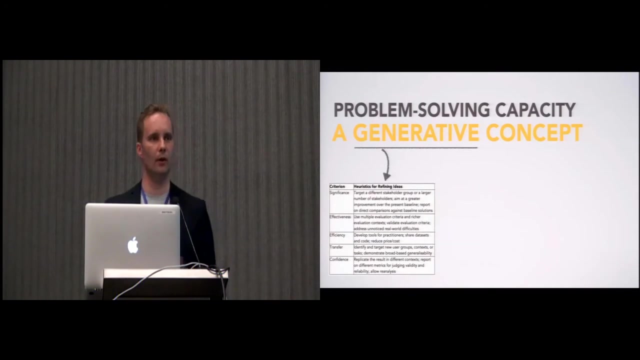 either the solution or the problem, ignoring the other, And this creates an imbalance. But we are not limited to just describing how things are. This can be used in a reverse manner, if you will, to generate ideas and refine ideas. So you can take the five criteria. 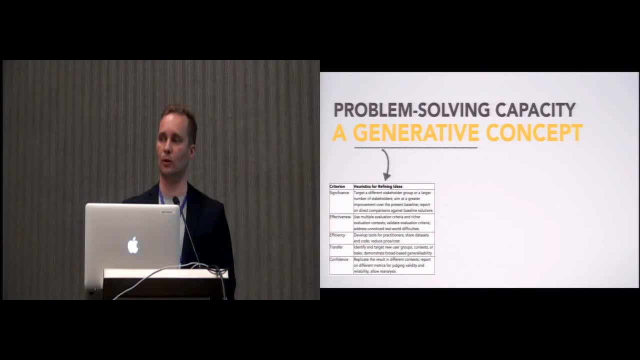 and you can generate heuristics or ideas on how you can improve your own work, And we offer a table in the paper that you can use as a starting point To demonstrate that it's of some value. we analyze Fitts' Law as a field. 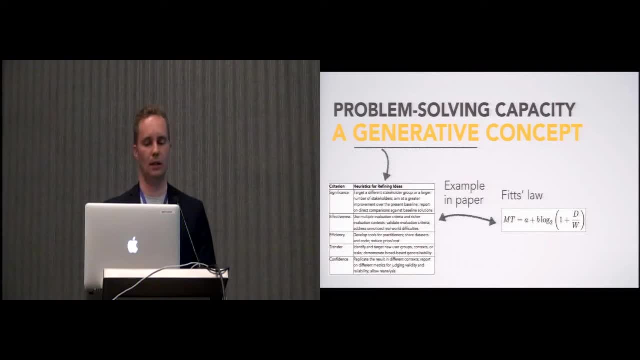 So it's a field that has existed for many decades And we could show that there are places where you can improve. There are basically goals that we can set for Fitts' Law research that make some sense. Of course, problem-solving capacity per se. 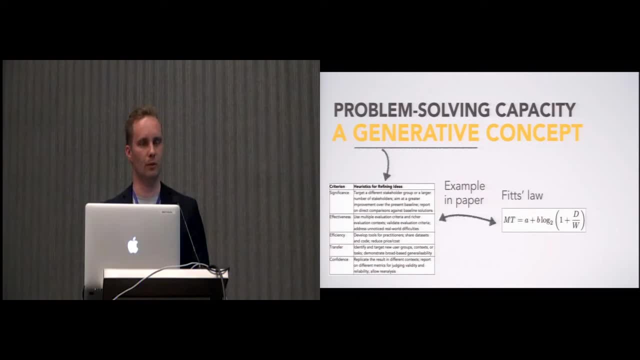 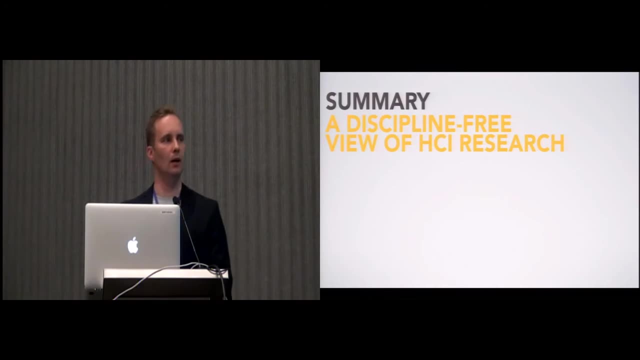 doesn't say how those problems should be solved. It's just saying that there's opportunity to improve our problem-solving capacity in that domain. Okay, to summarize, we're offering a discipline-free view of HCI research. It's a single concept. So if you only have limited capacity, like I have, 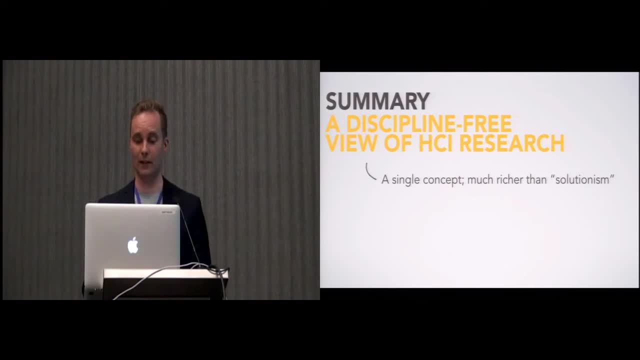 for attention, then this is a nice candidate for describing HCI, And I hope that I've shown that it's much richer than solutionism or your regular notion of problem-solving. It also embraces variety, without being naive, without making the fallacy that every perspective 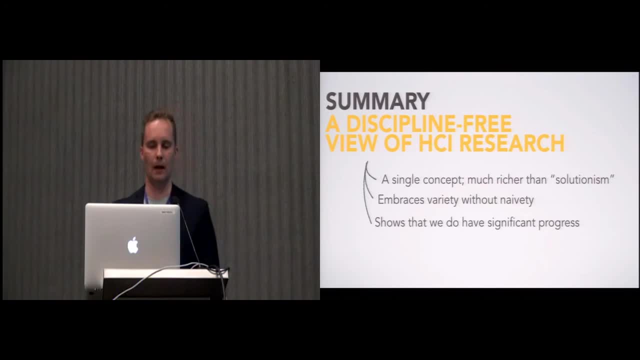 is valuable just because they're different, And it shows that we do have significant progress in our field. It's just limited into certain categories and it's not just about the number of people. It's about certain categories of progress And it shows that we have a need to work on. 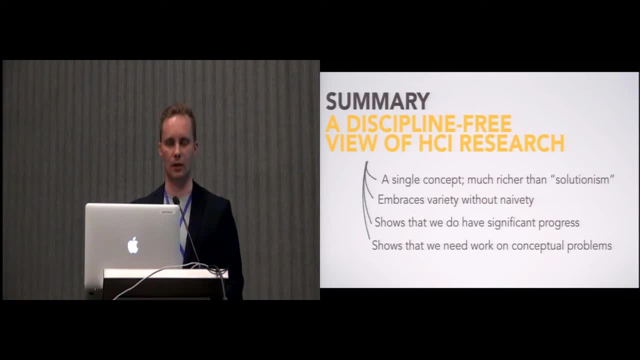 conceptual problems that can tie together empirical and constructive efforts. Finally, this is a full philosophy of science. You don't need to buy into that. You can use it also in a very pragmatic manner. You can use these tables and you can use these criteria. 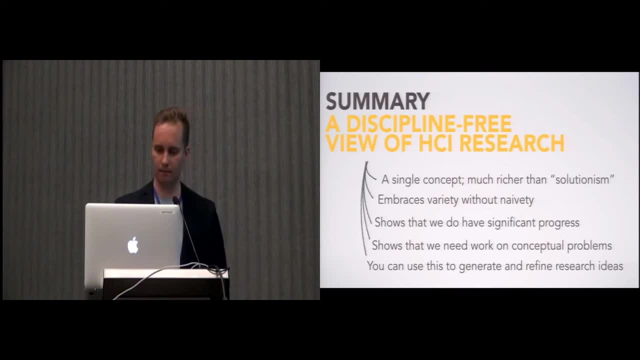 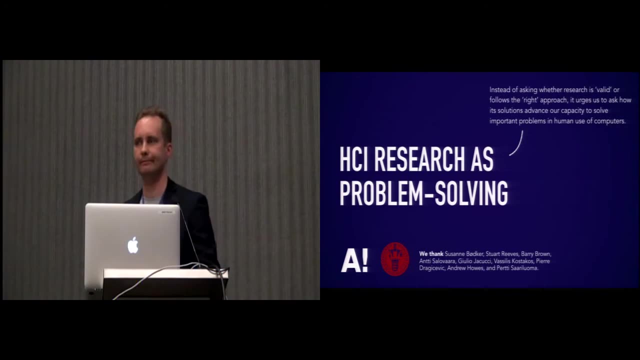 to refine your research ideas. Thanks, I'm very optimistic that there are some questions. Come on Hi. So I know that you talked about this idea of a problem as being an expansive idea, So you're talking about solving a problem. 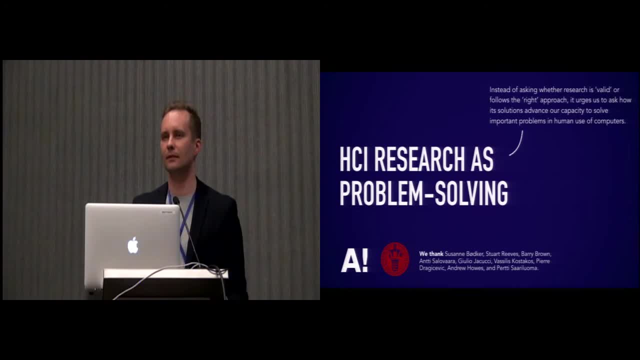 but I'm not sure that. maybe you can tell me how the idea. so it seems like not all research is about solving problems, right? So some research is about understanding themes or ideas, And one example is a paper here at this conference by Steve Benford was thinking about an idea. 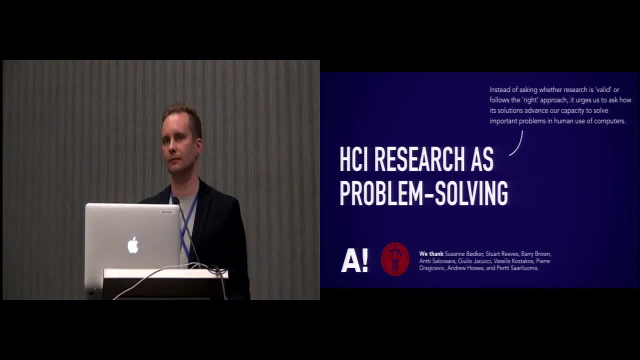 of accountable artifacts. That's not something that's actually like making a solution to anything. that's understanding a space. You're not gonna get to a final point. So how do things like that fit into this idea of problem solving? I didn't have time to go through all the subtypes. 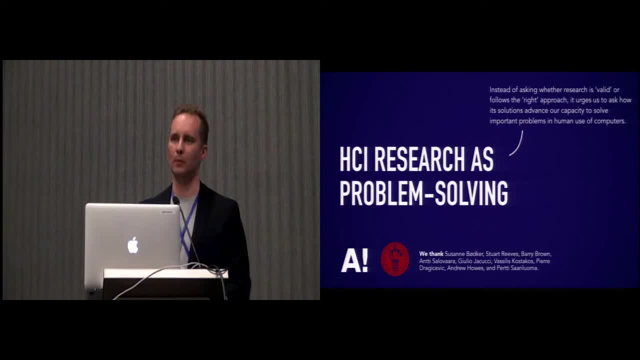 of each of the problems, but they always start with the subtype one, which is basically complete absence of a problem description. right, So it would count as a contribution like that, But I'm not sure it's ever going to get to a problem description. 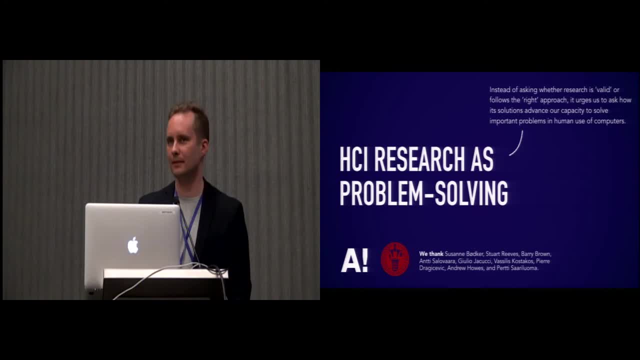 Sorry, I'm not sure it's ever going to get to a problem description. that's not the point. What is the point? Insight revelation illumination- That would count as subtype one. That's subtype. So Hi there, thanks for the talk. 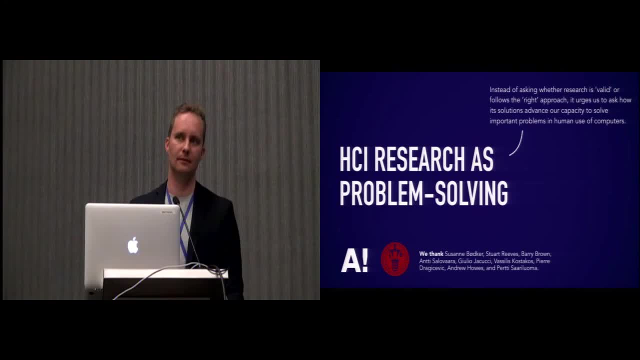 Sebastian Ditting from the University of York. I'm very much a pragmatist, so this kind of philosophy of science that to me kind of very much smells of pragmatism is right up my alley. Though my question is then, as a pragmatist: 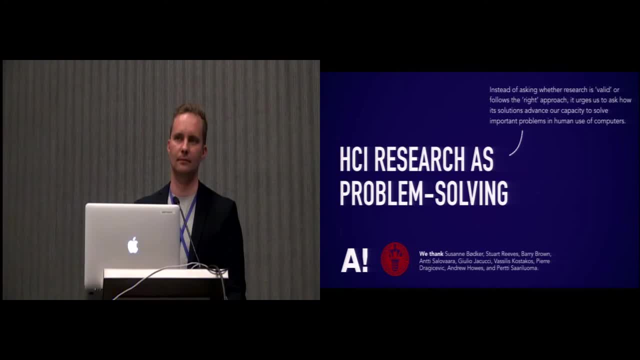 how does this change practice, and not just the way we talk about things? So how does this not just is yet another way in which we then write our introductions in our paper slightly differently in order to justify whatever it is we right now are interested in. 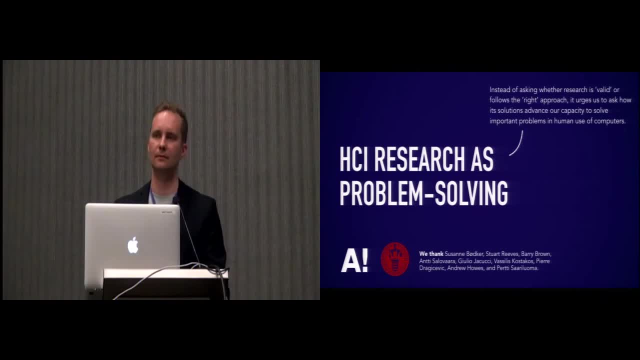 and whatever it is that we're interested in And whatever it is that we got money for. But how is this actually changing research practice? Yeah, I don't think there's any fast way to change the culture. Yeah, So it starts with individuals thinking differently. 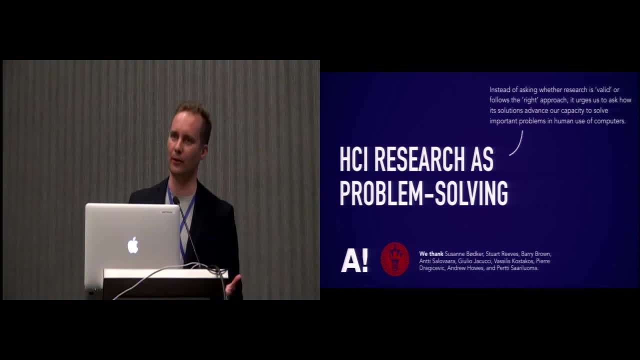 And then that seeps into their practices, And if they're better in their own work, then others will copy them and maybe it will distribute like that. We are using this in our lab and it seems to work there. Okay, So the proof is in the pudding that your lab 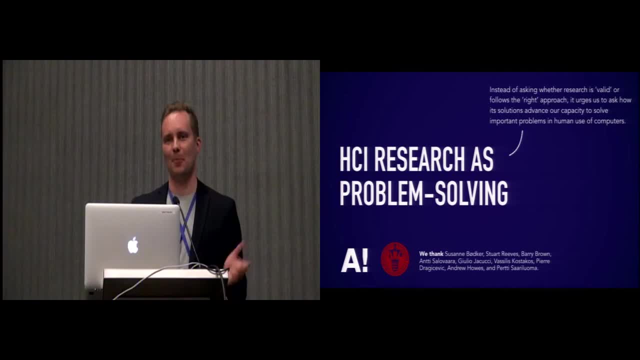 will be so much humongously more successful that everybody will follow on the bandwagon. Now we have 300 people in the room, so let's see this here. Okay, thank you, Very nice work. You've abstracted away the method. 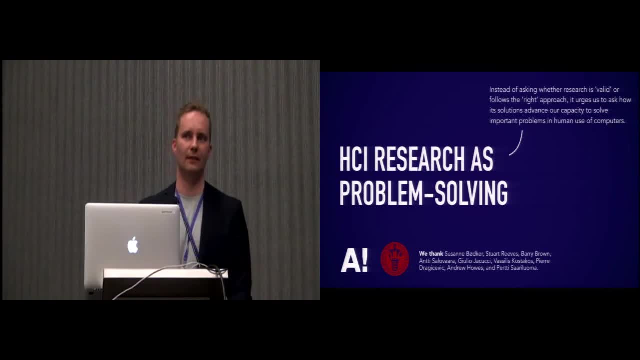 and I understand why you abstracted that away. but of course, in order to judge the solution, we need to judge what the method was. So can you talk a bit more about that distinction, like: when does the method come in, or is it the right, suitable method for a particular problem? 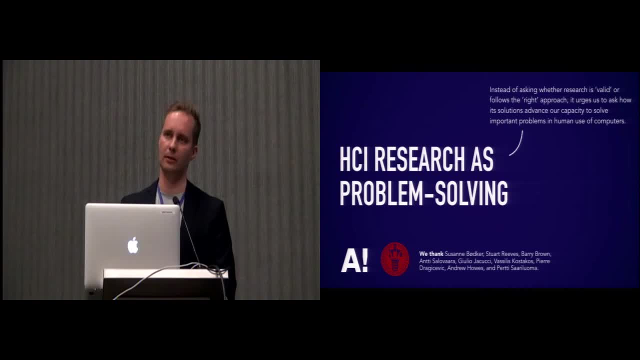 One of the criterion was confidence, right. So you would evaluate the method in terms of how probable you hold that this problem solving capacity that you claim holds. So then you would evaluate basically the methodology of that. So it would be part of the evaluation.